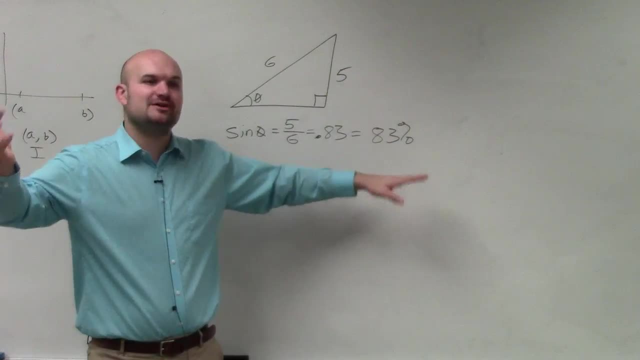 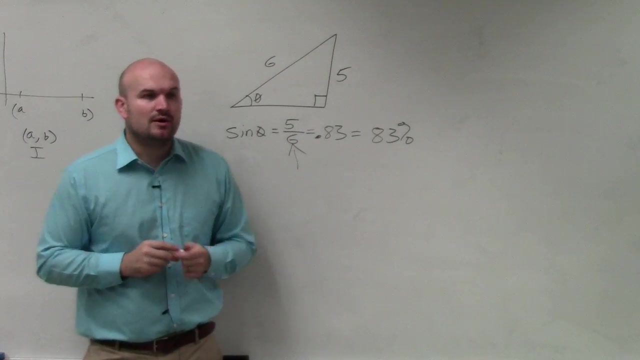 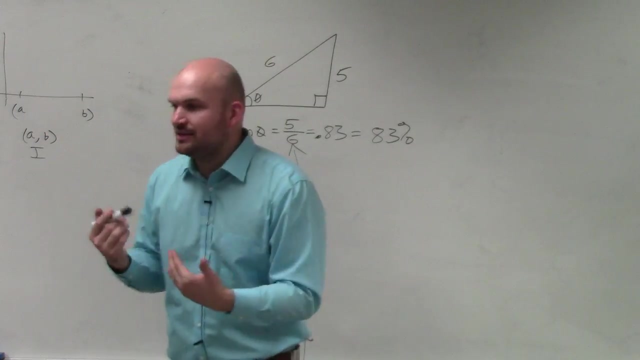 I am. I'm using the 83% as a understanding measure, but if you remember, on the last quiz, I wanted you to leave everything in fractional form, right? So, yes, your understanding of 83% would like make sense. sense, but basically what we're looking at is leaving everything in like our fractional form. Yes, 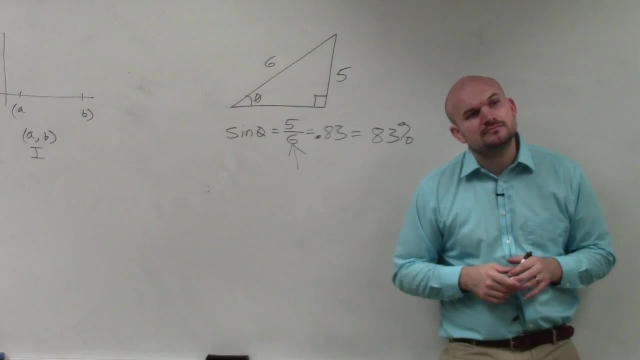 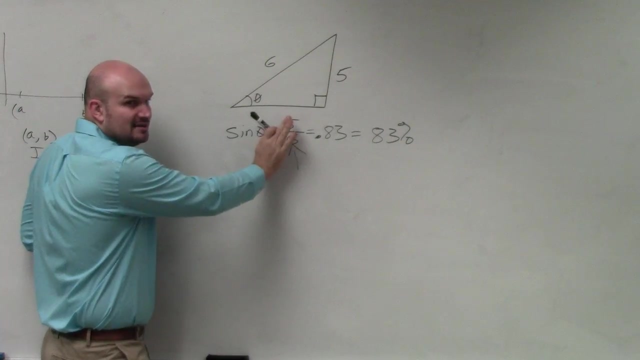 How do we convert the decimal form to the fractional form, or is that not? Yeah, but you? the only way to get to your decimal form? for me is you had to divide 5 or 6. you just leave it like that. this is more. 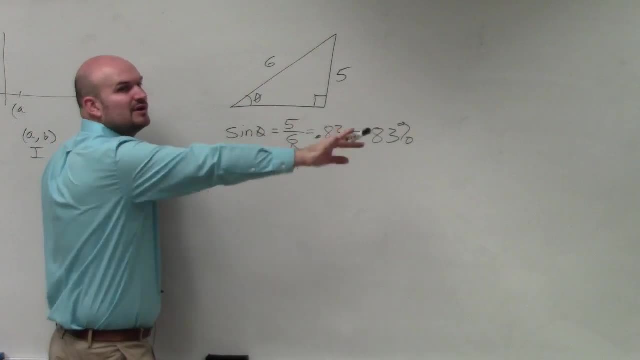 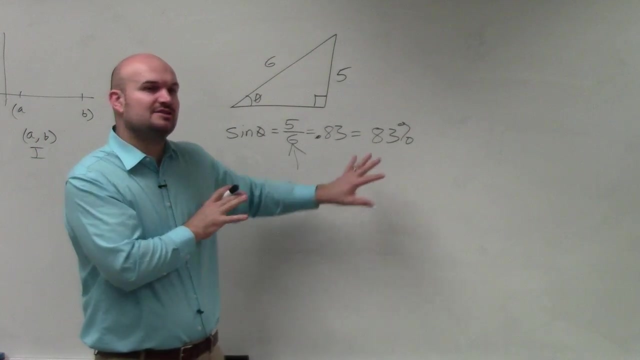 work. you just have 5 or 6, that's it done. you don't have to go any further. I'm gonna go over what we're gonna cover in class. I just wanted to. I mean, I'm gonna go over problems that you would see so you'll understand how to leave the. 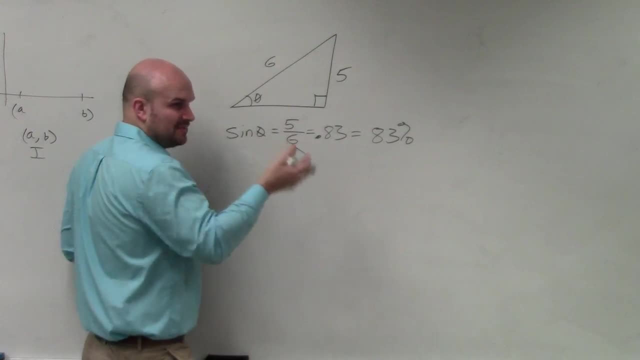 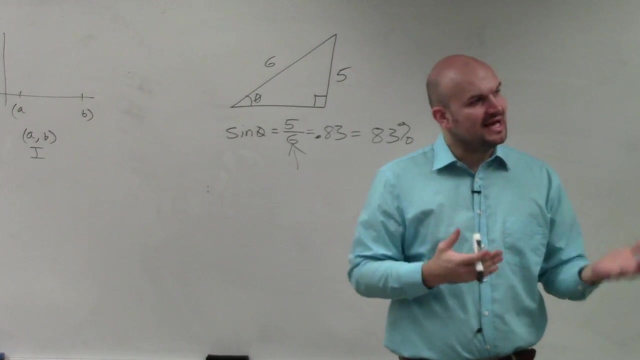 answer. my main point of thing is: everybody remember sine and cosine, which is correct. sine is opposite over hypotenuse, cosine adjacent over hypotenuse, tangent, opposite over adjacent. but again, a lot of times when we get, we're gonna start getting answers as decimals and I want everybody to kind. 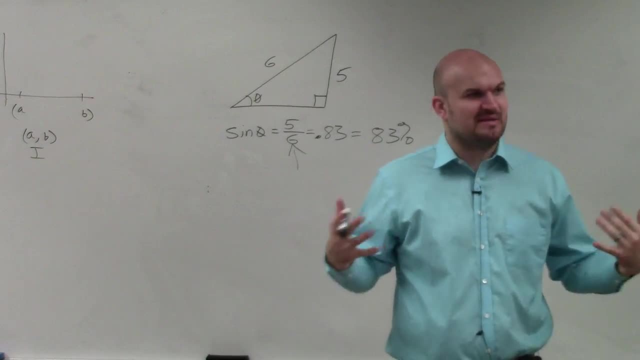 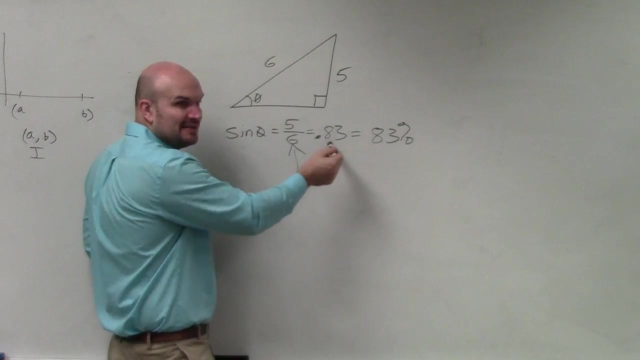 of understand, like: what exactly do these decimals mean, rather than just hey, here's my answer. as a decimal. well, if you get a decimal and you get sine of some angle is 0.83, right, let's? let's just forget about all of this, let's just 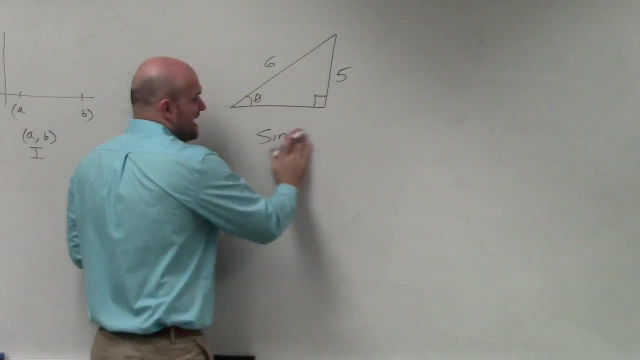 pretend. my answer is: you know, I do sine of some angle, whatever that angle is, and I get 0.83. conceptually, what does 0.83 mean? oh, of whatever angle. let's just say it's 36 degrees, right, and we're gonna do problems like this. but what if? my answer 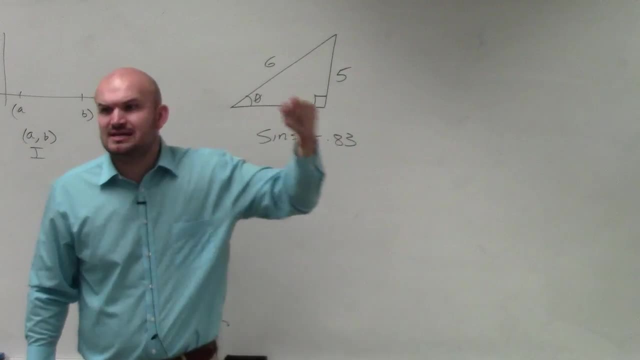 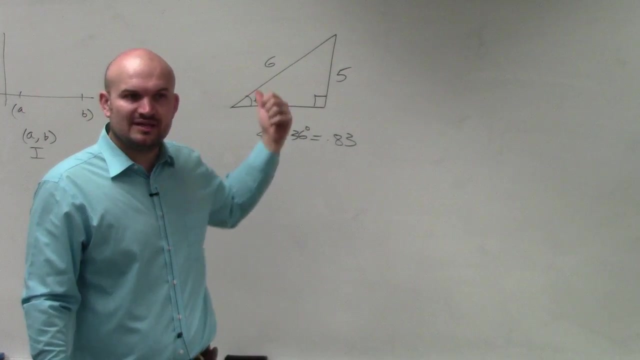 sine of 36 is 0.83 conceptually. what does that tell you? oh, a triangle at 36 degrees means the opposite side is 83% of the length of the hypotenuse right, so I'm not using it, as this is what you're gonna do for a test or around a quiz. I'm 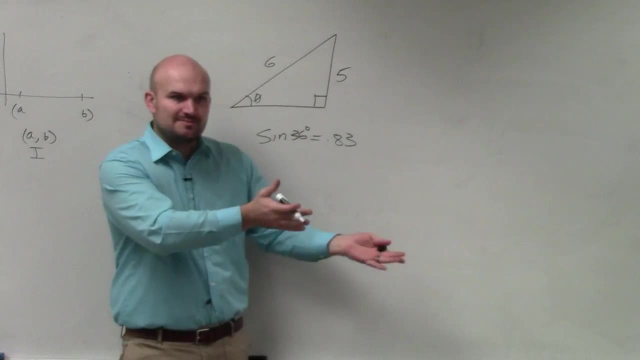 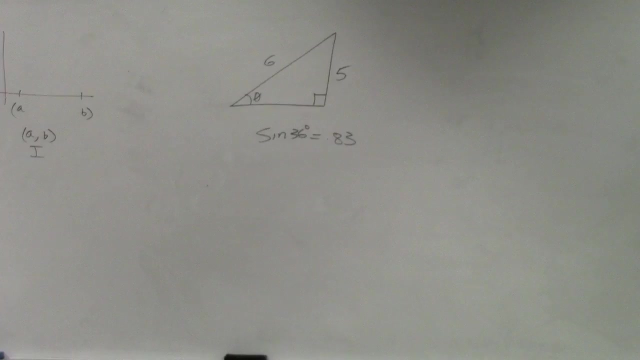 just doing it for your conceptual understanding of getting these decimals, because it's Stallảnh. that's what we're going to kind of move into next. all right, So my example that I wanted to work on: